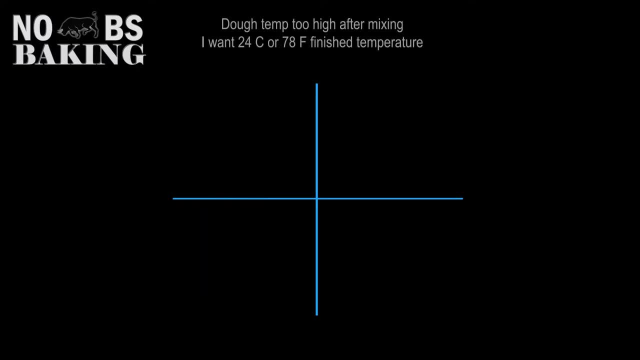 So now let's look at a few examples. In this first example, we followed an online recipe and used 21 degrees Celsius water, But our dough temperature came out too high, at 32 or almost 90 degrees Fahrenheit. We want to adjust our water. 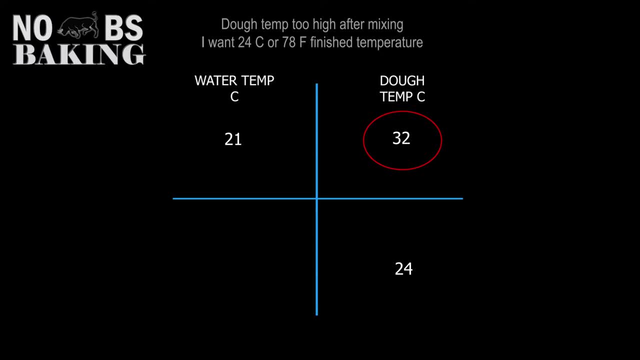 temperature for a dough that, with the same ingredients, the same mix time, will finish out about 24 or about 78 degrees Fahrenheit. So here's how we do the math: 24 times 21, divided by 32, and our answer is 16.. We need 16 degree water for this. 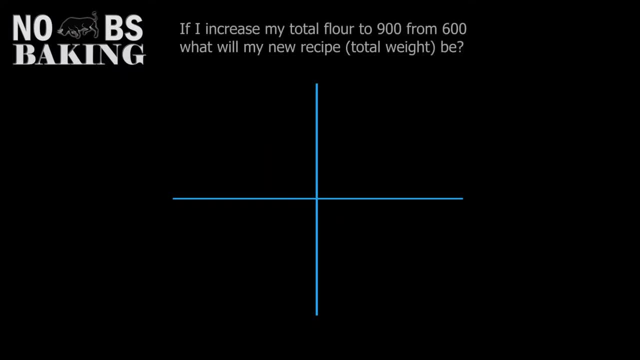 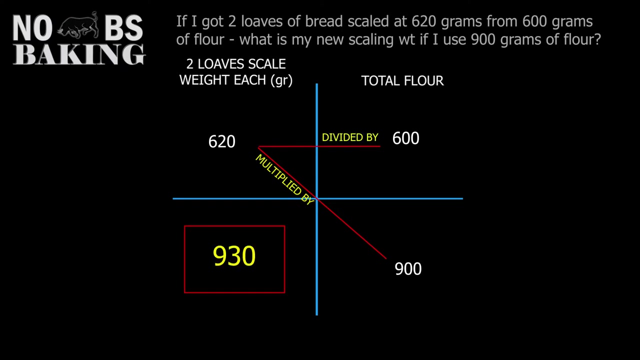 dough. Now here are just a few more examples. Take your time, walk through them, work them out on paper and you can see how easy ratio and proportion is. The first time we work with 24 degrees Celsius water. we start with 24 to get. 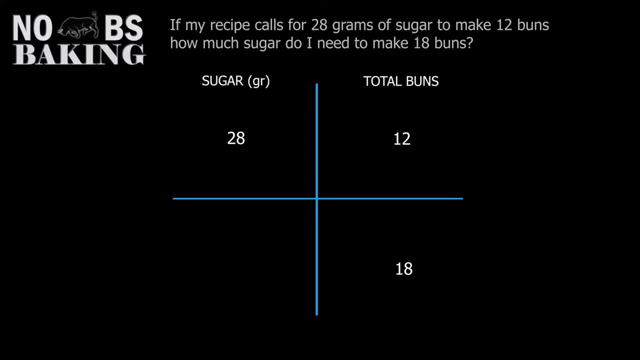 what we're doing. So we try and keep the water at a medium temperature and we keep beating it until it reaches 27 degrees Fahrenheit. We're now going to make the dough into an orange. So we're gonna take the white egg yolk and we're going to add that to a dough, We're gonna add our flour and we're 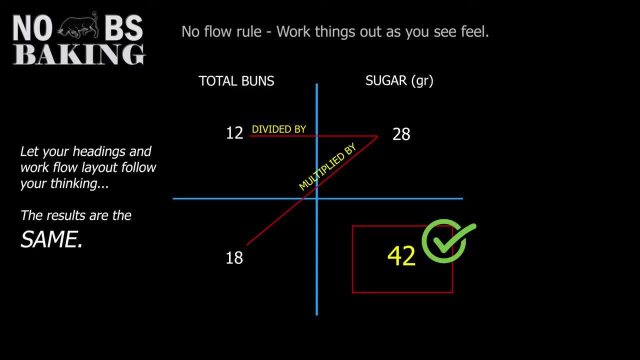 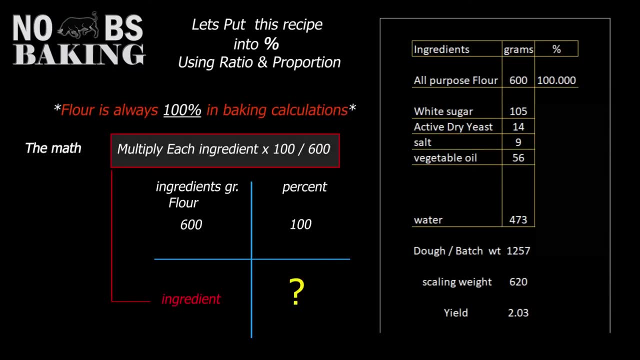 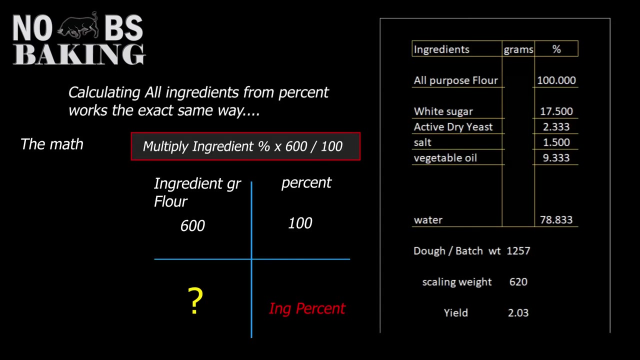 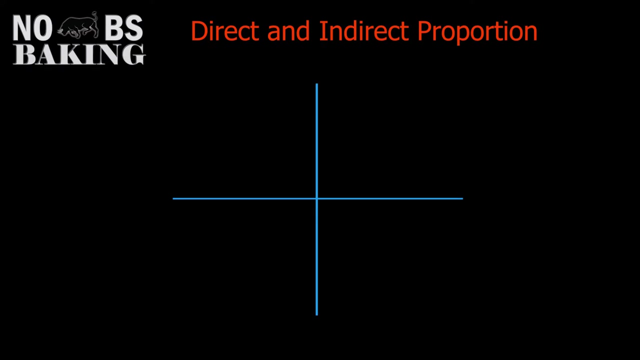 going to use our hand blender to mix it. Thank you. Until now we've looked at direct proportion, but now we're going to look at indirect proportion. So your bread's coming out too slow. your room is warm enough, but the dough is taking 90 minutes to final proof. 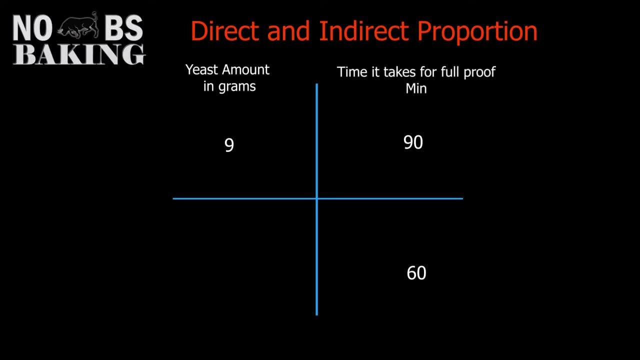 when you use 9 grams of dried yeast. Now you want to increase your yeast to give you closer to 60 minutes of a final proof time. So you lay your headings out, you do your math and the number comes out to 6..